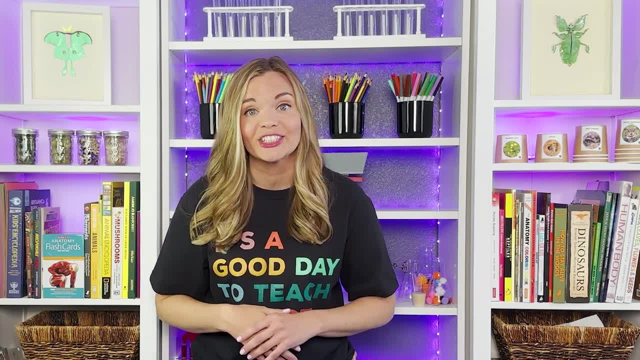 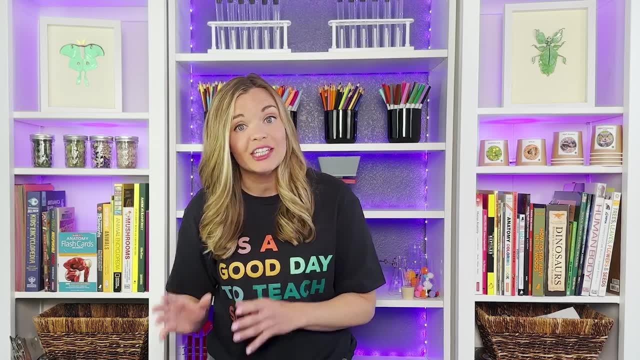 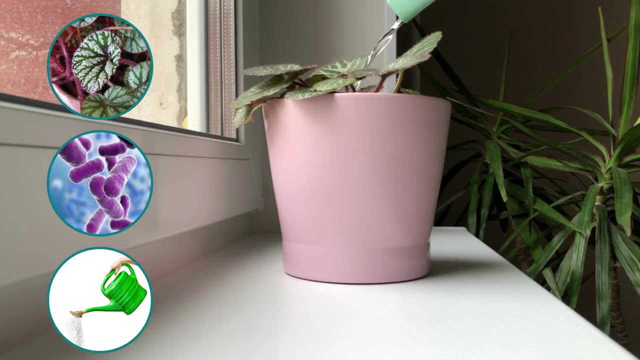 it will contain both biotic and abiotic factors. For example, a houseplant growing on a windowsill may be considered a small ecosystem. Biotic factors include the plant, the bacteria or organisms in the soil and the human taking care of the plant and keeping it. 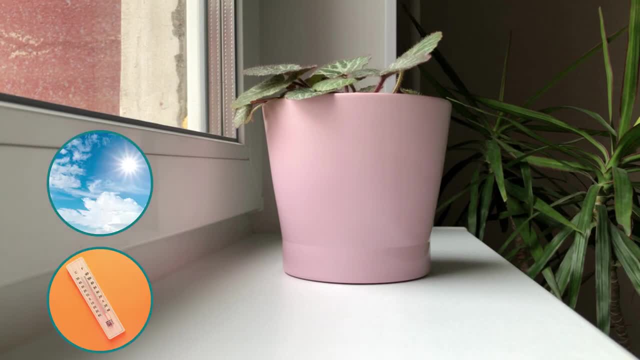 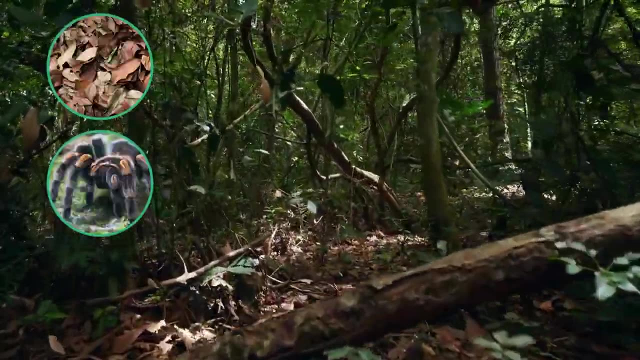 alive. Abiotic factors include light, the temperature, the soil and the pot. In this rainforest, the biotic factors are the dead leaf litter, the spiders hiding underneath the scurrying lizard and the tree that it's on, and the lichen growing on the branches. 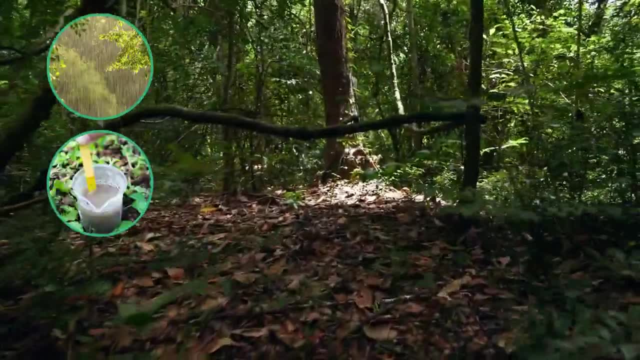 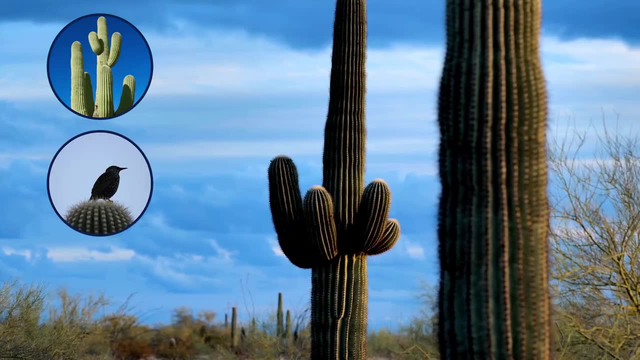 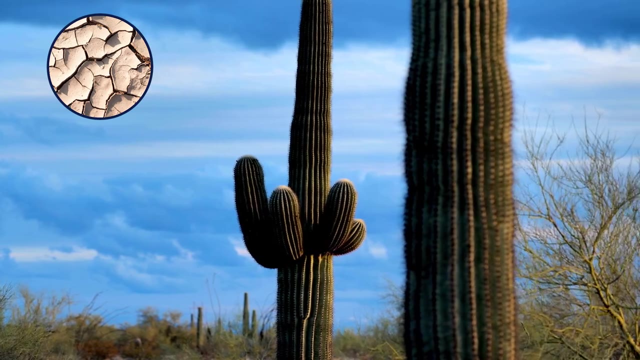 Some of the abiotic factors are the rainfall and the pH level of the soil. In this desert, the biotic factors are all the cactus, the bird living inside and the scorpions hiding under rocks. An abiotic factor would be the lack of humidity or the dryness of this ecosystem. 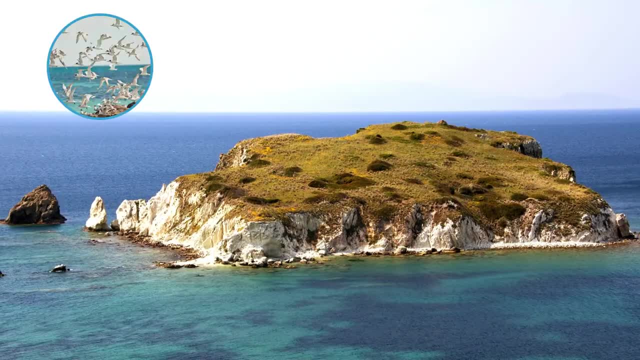 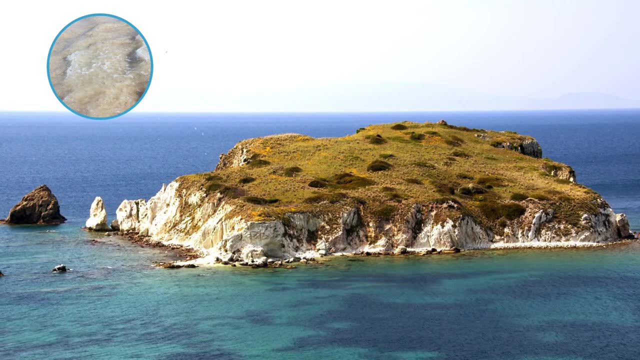 On this tiny island. the biotic factors are the seabirds and the seagrass growing on top. abiotic factors are the water and the soil and the scorpions hiding under rocks. Abiotic factors are the salt content of the water and the erosion action of the tides and waves. 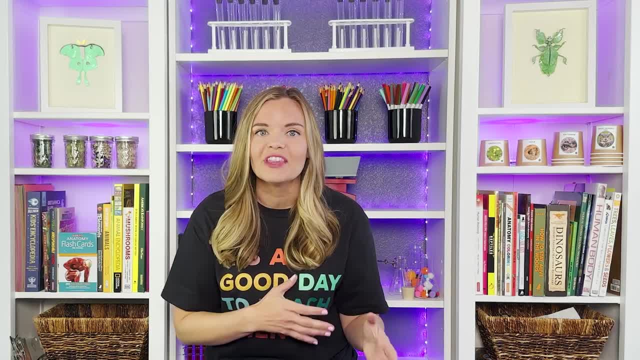 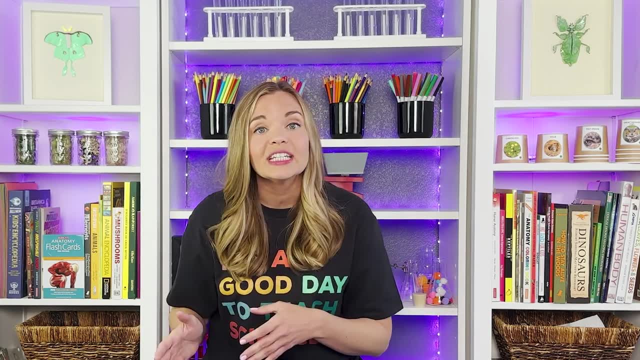 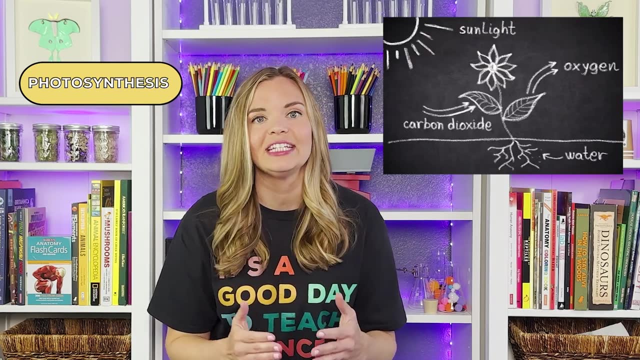 To survive, these biotic factors need all of the abiotic factors. Even slight changes in abiotic factors can have a significant impact on the organisms in an ecosystem. Photosynthesis is a great example of abiotic factors such as sunlight, water and the chemicals in the air working together 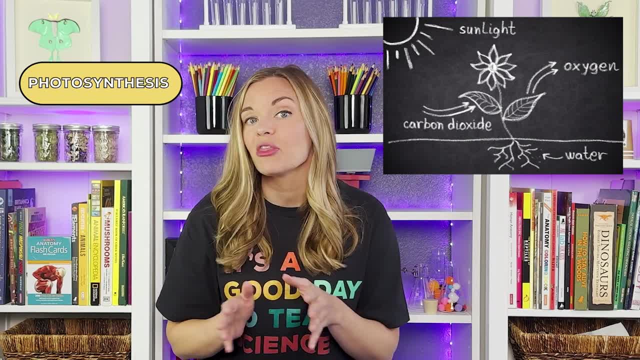 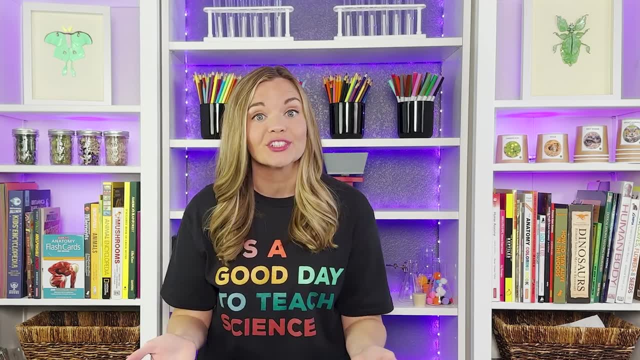 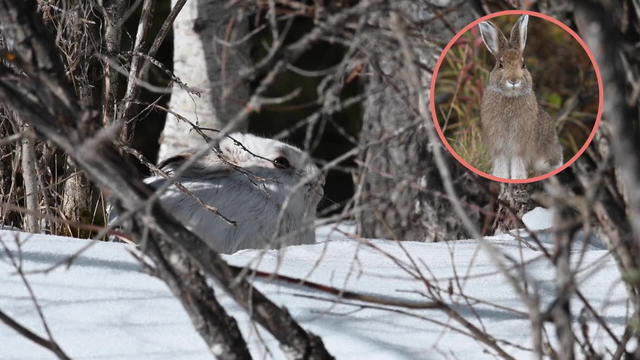 with a living organism or a biotic factor: the plant. This is really important because every food chain or food web begins with plants or producers. This snowshoe hare changes the color of its fur as its environment changes to help it camouflage and avoid predation. 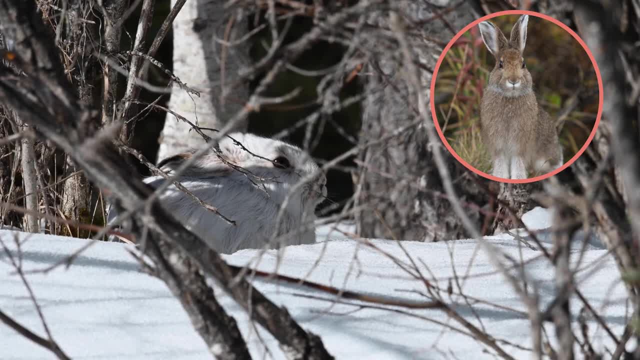 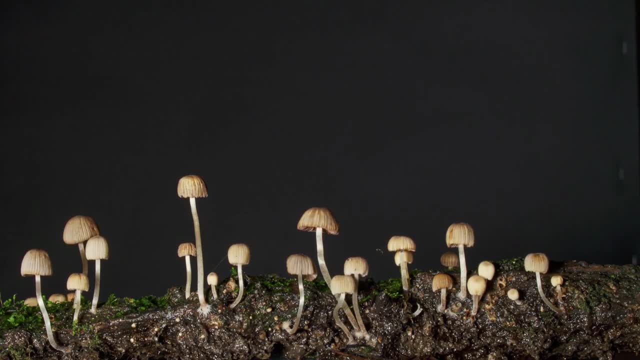 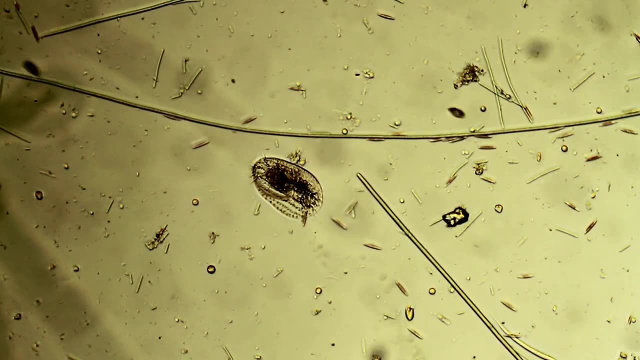 The white snow is an abiotic factor that causes the hare to grow different color fur, so it's more successful in the environment. Bacteria, fungi and microorganisms in the soil change the chemical composition. Algae and microorganisms in pond water change the oxygen level to make the water more or less hospitable to other organisms.